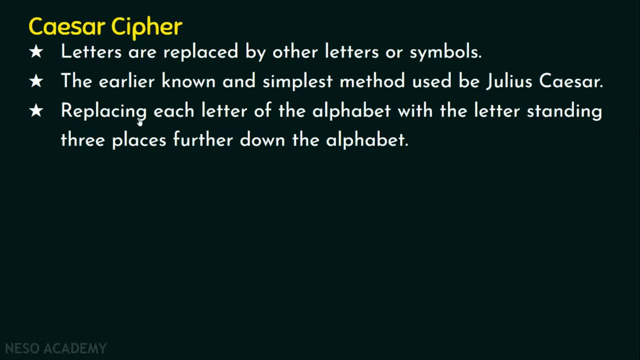 We are going to take 3 places further down the alphabet, the plain text letters, and we are going to replace each letter of the plain text and that alphabet is going to be substituted by the alphabet three places further down the alphabet. Don't worry about this. now, When we see an example, you will understand this point clearly, So we can confirm. 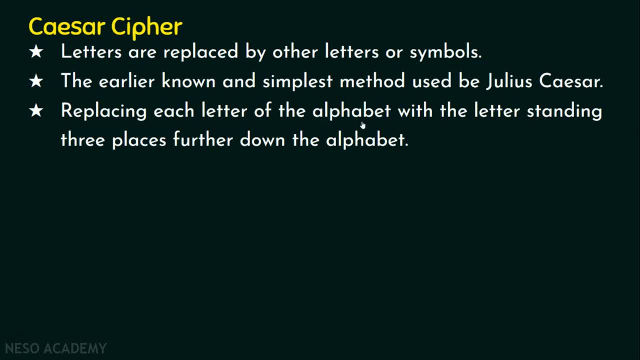 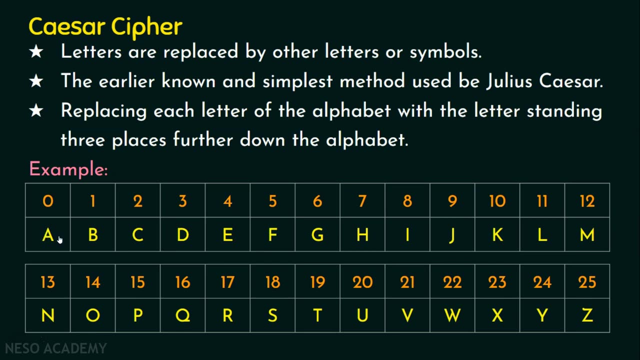 from this point that we are going to replace each letter of the alphabet with the letter standing three places further down. So we need the alphabet right. So we will take the example. Here is the list of alphabets in English: A, B, C, D and up to we have Z, and can you notice here? 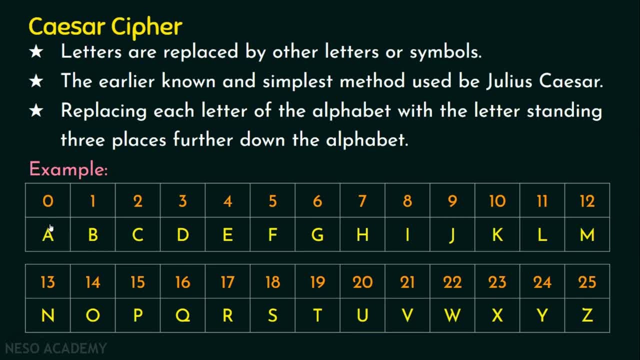 each alphabet is assigned with a number starting from zero. So A is assigned with the number zero, B is assigned with the number one and C is assigned with two, and so on and so forth, and finally we can see: the alphabet Y is assigned with 24 and the alphabet Z is assigned with the. 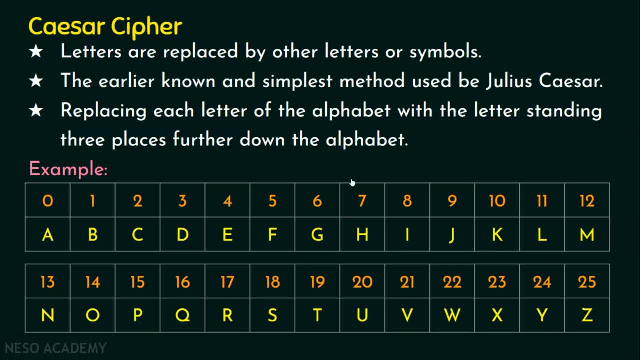 number 25.. Since we have 26 alphabets and we have started the alphabet from the number incansable, we can say A is assigned with the number zero and B is assigned with the number 25.. Now let's see how to do this. So let's start with the alphabet in English. Let's see: 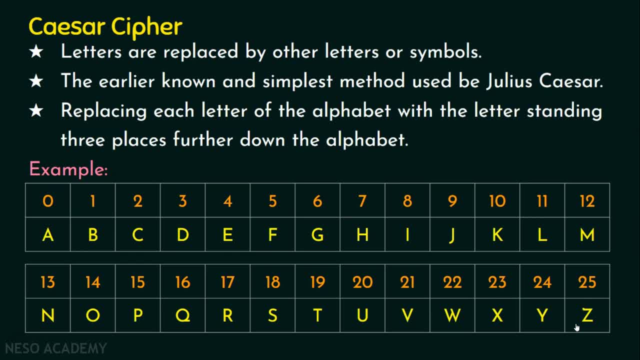 0.. So it ends at the number 25 for the alphabet Z. So please make a note of this. You can start with 1,, 2 or 3.. I am talking about the method which was used by Julius Caesar, and that's why. 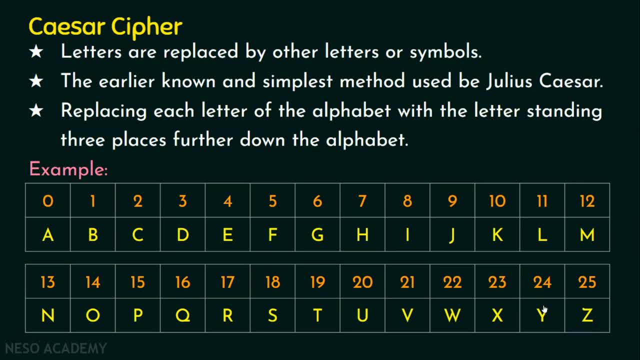 this technique is called as Caesar cipher. We will see an example how encryption is done. So in this encryption technique the plain text letters are going to be replaced 3 letters further down. Suppose: if we want to encrypt A, so A is going to be replaced by 1,, 2, 3.. So A is going. 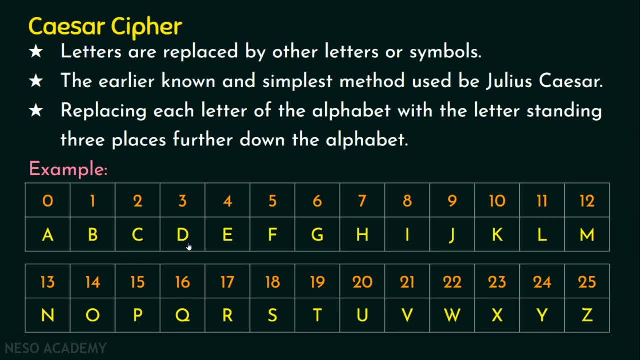 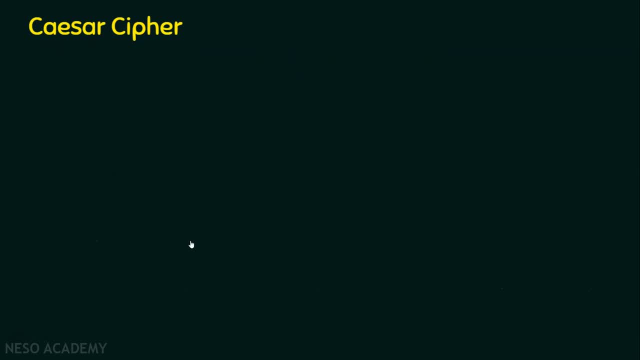 to be replaced by D. Likewise, all alphabets are going to be replaced by 3 places further down the alphabet. So before seeing the example, let's see the algorithm. now The algorithm of Caesar cipher is simple. For each plain text letter P, we know P is the plain text and substitute the cipher text. 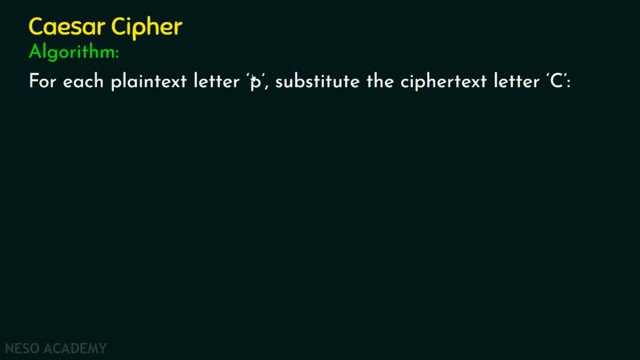 letter, capital C. Can you see here the plain text? In this example, it is going to be represented in lower case and the cipher text is going to be represented in upper case, and that's why we have used a symbol like this. It's not mandatory, but 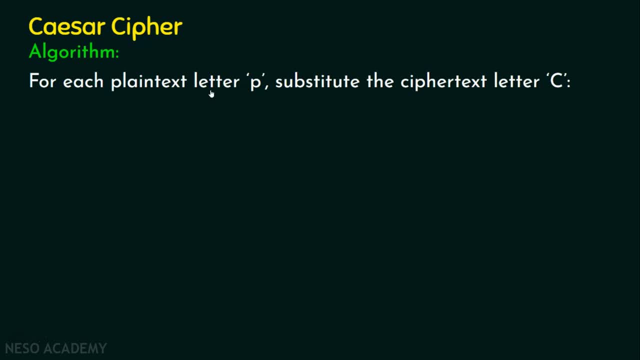 it gives elegance when we do like this. So the algorithm states that for each plain text letter P, we are going to substitute the cipher text letter C, Say in the plain text. if we have multiple characters, we are going to encrypt all multiple characters by other characters, right? 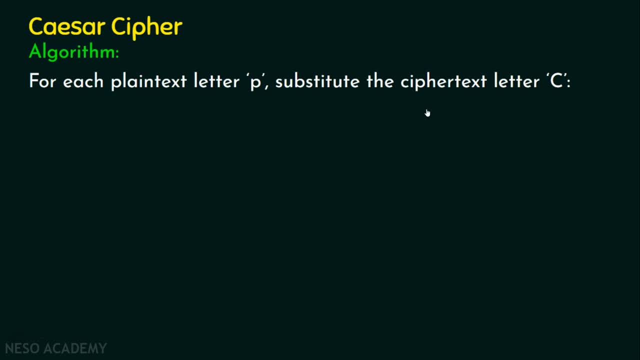 So as a whole we are representing the plain text letter with P and cipher text. How cipher text is generated: We know cipher text is going to be the output of the encryption process. We know what encryption is going to do. It's going to take two inputs, right? 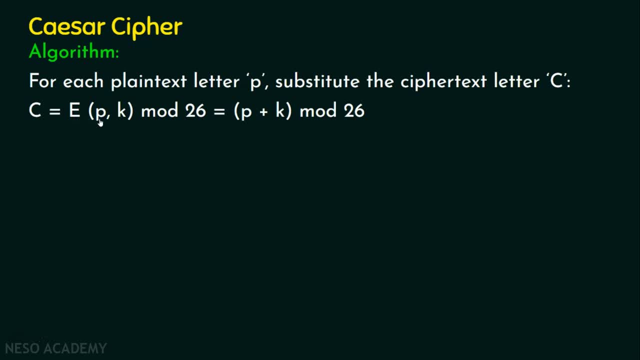 Any encryption algorithm is going to take two inputs. Number one is the plain text and the other one is the key information: How many places we are going to progress in order to get the cipher text In Caesar cipher. we have seen three places right, So here the K is. 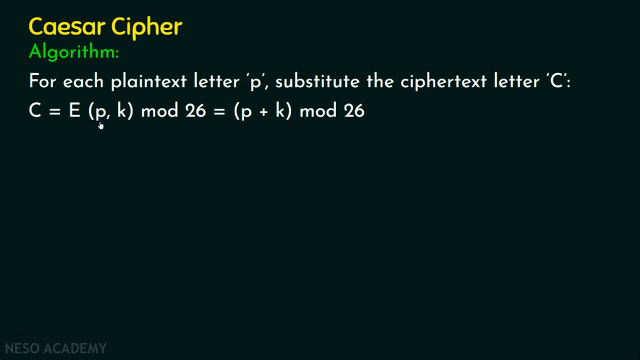 going to be 3 always. So we are going to take the plain text as the input and K is the key which is given to the encryption algorithm, and this encryption algorithm is going to generate the cipher text right, And we are going to perform the mod 26 operation. 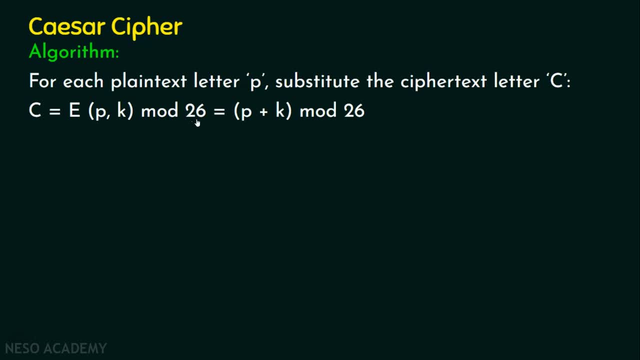 Why we want to do mod 26? I'll explain that when we see an example, Since we have 26 alphabets in English, and this is mainly for English language, and that's why we are going to use mod 26.. So what is the operation actually? How cipher text is generated. Just take the. 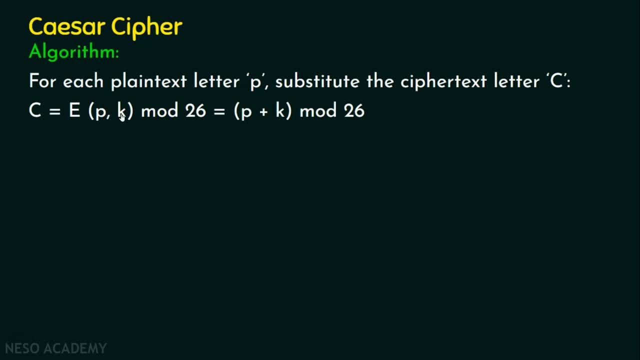 number pertaining to the plain text character or the symbol. Add that with the key. So just take the number pertaining to that plain text letter, Add that with the key. Here key is going to be 3 because Caesar cipher is going to work with the key value 3.. I already 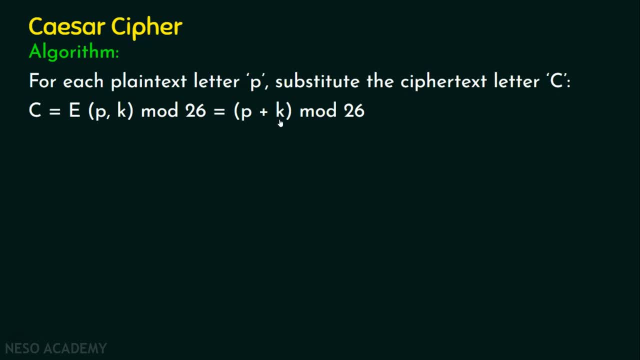 told you how many places we are going to proceed with, or further down. It's going to be three places, right? So plain text value plus 3 mod 26. we need to perform Why? Because we may be encrypting the last characters also, right, It may be Y or Z, So in that case, 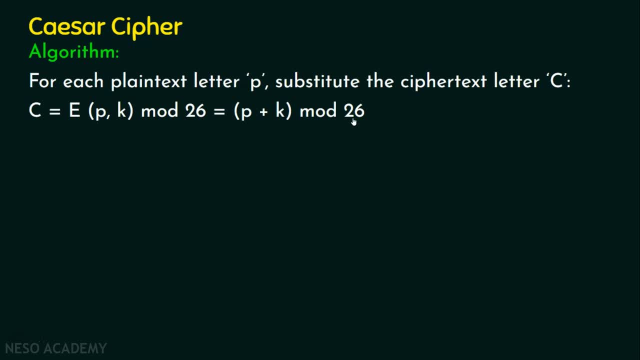 it should not go out of the range, and that's why we are performing mod 26.. And this is about encryption. and what about decryption? So we know, in the encryption process the plain text is given as the input and key is also given as the input, and then 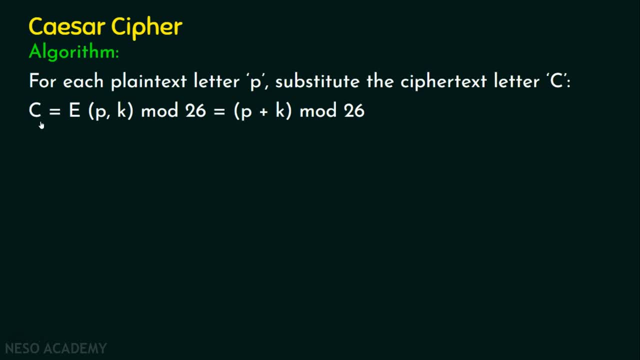 we get the cipher text, But in the decryption it is the reverse of encryption right. So in the decryption we will be getting the plain text back, But this decryption is going to take the ciphertext as input and also key as one of its input. 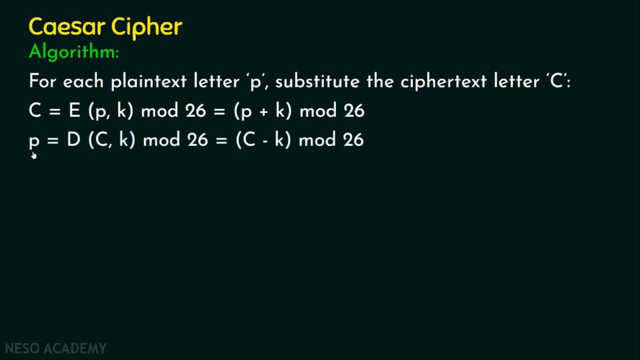 Let's see that now. So the output of decryption is going to be the plain text back, But this decryption algorithm is going to take the ciphertext and the key and we are going to perform mod 26.. As I mentioned, it is the reverse of encryption, right? 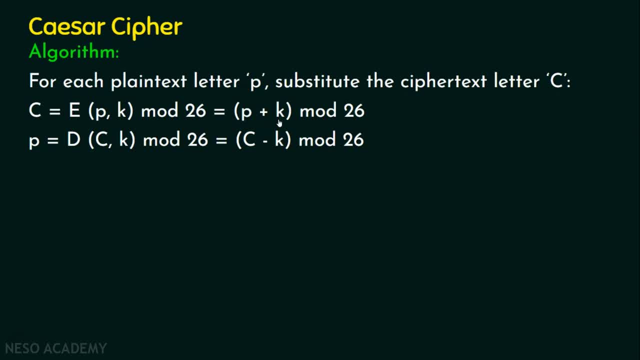 For encryption we are going to take the playing text letter's number plus key, But here the ciphertext number minus key and we need to perform mod 26.. So this is the algorithm pertaining to Caesar cipher. Say, if we want to encrypt the playing text letter e. 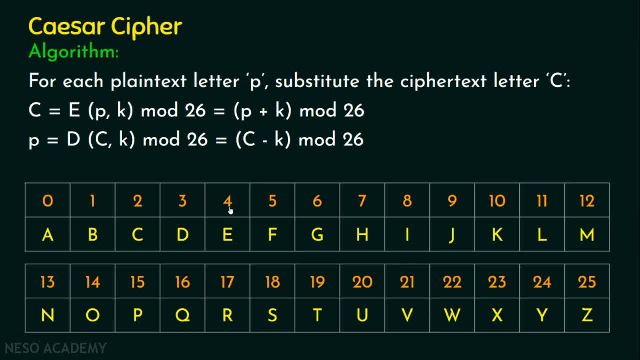 just take what is the number pertaining to this letter, e It is 4, right, So just add 3 to this 4.. 4 plus 3 is what 7.. So for the playing text e whatever is there in 7,. 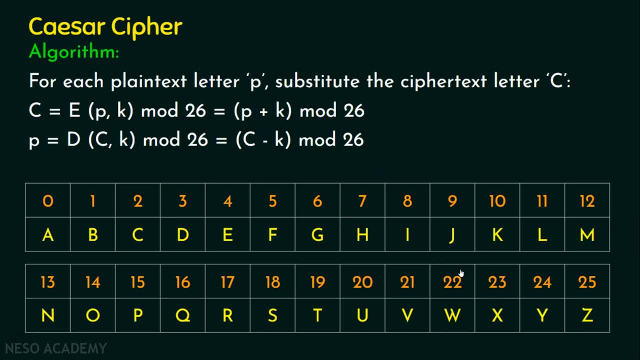 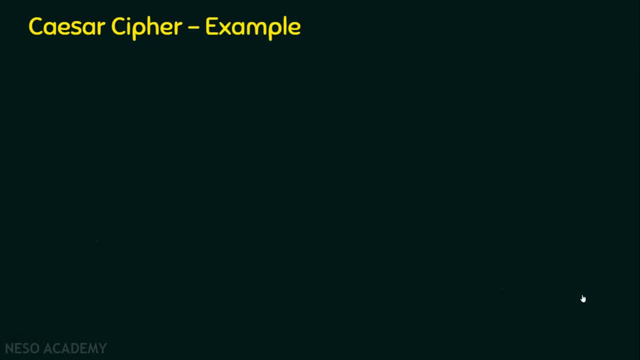 that is the ciphertext, right? We need to perform mod 26 in case, if it is going with this value, like 23,, 24 or 25.. No worries, let's see the example in order to understand things better. Let's see the example now. 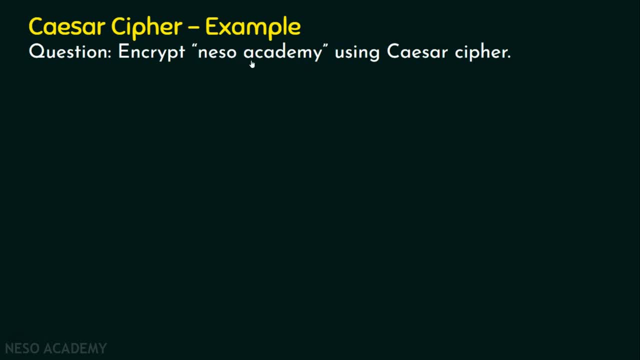 In this example, we are going to encrypt Neso Academy, which is the playing text, using Caesar cipher. What is the key value? By default, Caesar cipher uses the key value 3, right. By keeping that in mind, we will solve this problem. 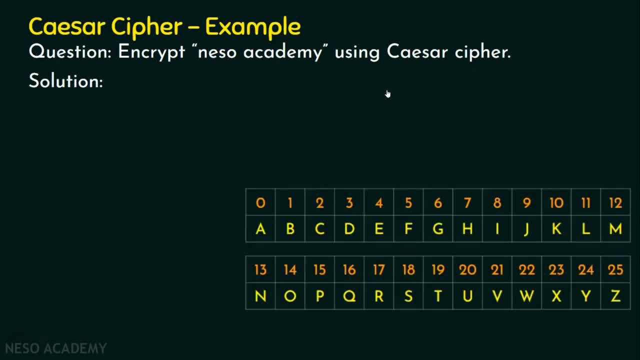 To solve this question. I am using a different approach, So we need this table in order to do this right. We need this table and for solving this, I have taken two row approach, where, in the first row, I am going to use the playing text. 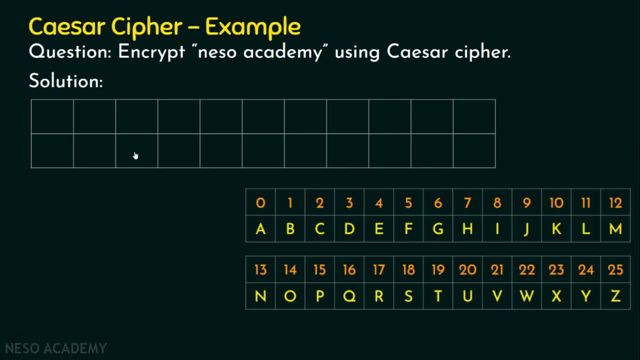 and in the second row I am going to generate the ciphertext, right? So what is the playing text which is given in the question, Which is Neso Academy? So I am going to fill that in the first row. Neso Academy is filled in the first row. 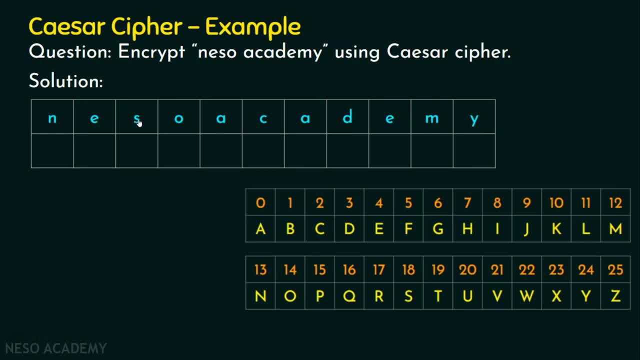 and we are going to generate the ciphertext for every individual letters of the playing text, right? So we will solve that. now Let's start with the first letter N. It means we are going to do encryption for the first letter N, So we know the formula for encryption is. 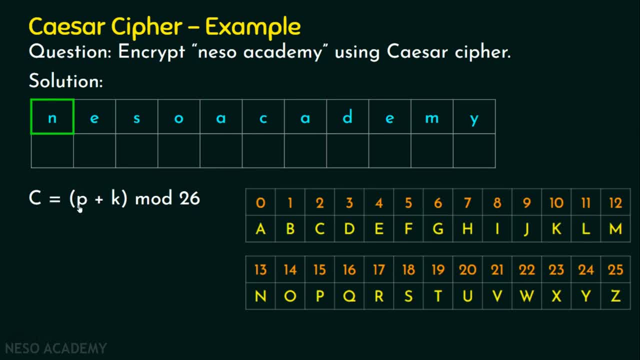 ciphertext will be the output. We are going to take the playing text position value plus the key mod 26.. What is the playing text position number for N? Just go and see the table. N is 13,. right, So I am going to use the p-value as 13 for N here. 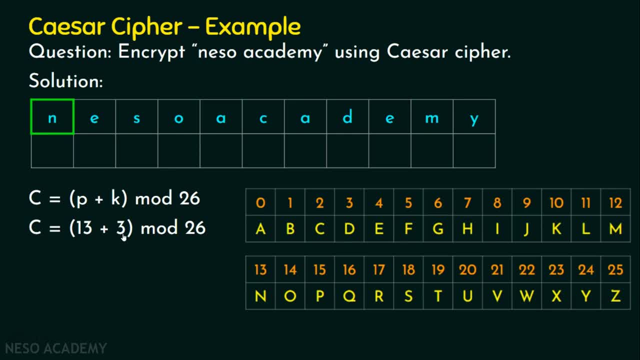 because N means it is 13. So 13 plus we know in Caesar cipher the key value is 3 mod 26.. And this is a simple addition. So 13 plus 3 is equal to 16, 16 mod 26.. 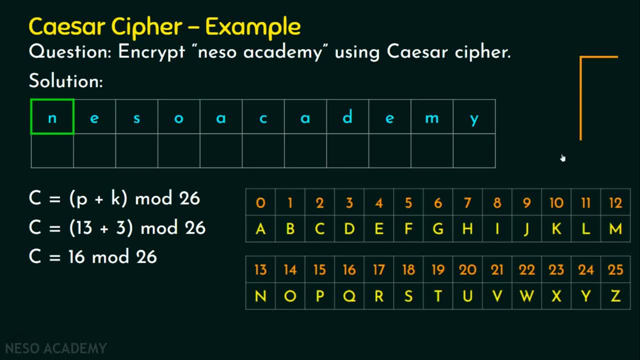 So the normal mathematical operation I am going to perform, just look at here the mathematical operation where 26 is the divisor and 16 is the dividend. So 26 is the divisor and 16 is the dividend. How many times this 26 can take upon 16?? 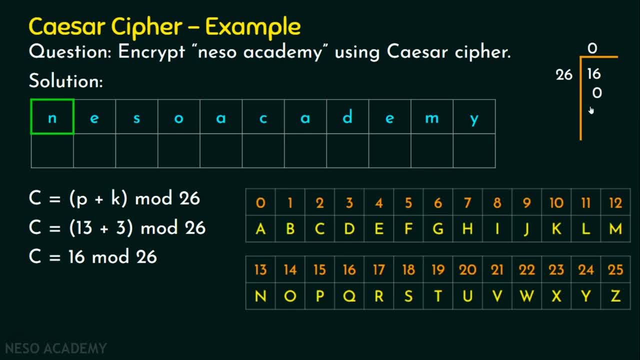 Zero times right. So 26 zero times zero and we get the remainder as 16.. So 16 is the remainder. So always remember the output of mod operation is going to be the remainder, not the quotient right. 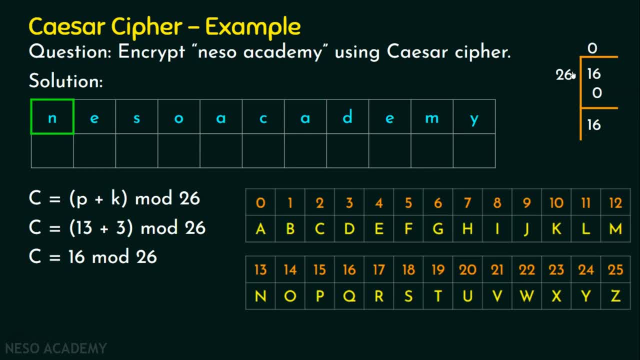 So what is 16 mod 26?? So when 16 is divided by 26,, we get the remainder as 16.. Now, 16 is the answer for this ciphertext. So what is 16?? What is the letter equivalent to 16?? 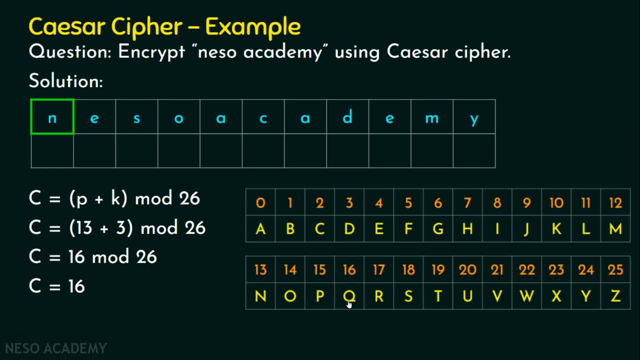 In the table, if you refer, the equivalent character for 16 is Q. So N is encrypted as Q, Can you understand? So the ciphertext is what Q. So this is the equivalent ciphertext letter for the plaintext letter N. 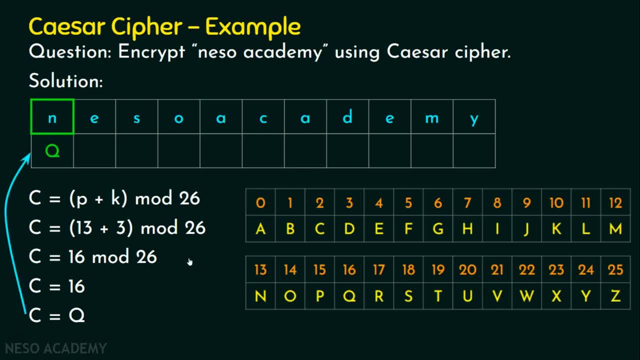 So this Q is going to be placed in the second row's first place. So N is encrypted as Q. Let's solve the second character, which is E, So we can easily do it. We know the formula for generating the ciphertext is: 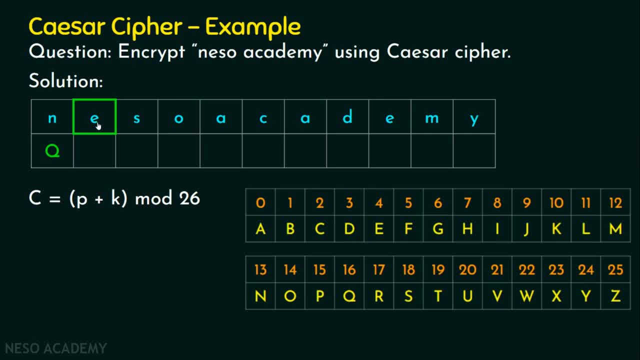 P plus K mod 26.. What is P value Here for E? the plaintext value is for E, it is four. So just use four plus the key value, three mod 26.. Four plus three is seven, Seven mod 26.. 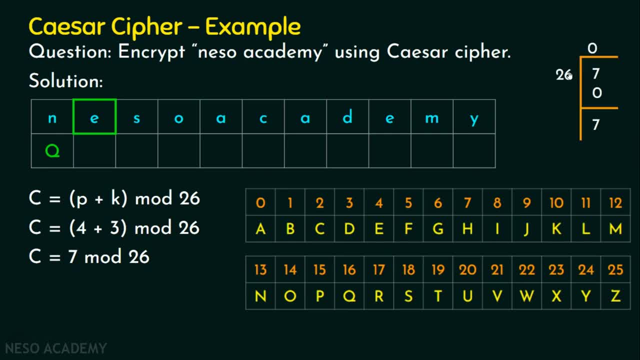 Just divide seven by 26.. So seven, when it is divided by 26, zero times zero, the remainder is seven, right? So seven is the answer for this equation. So the ciphertext letter is equal to seven. What is the character present in seven? 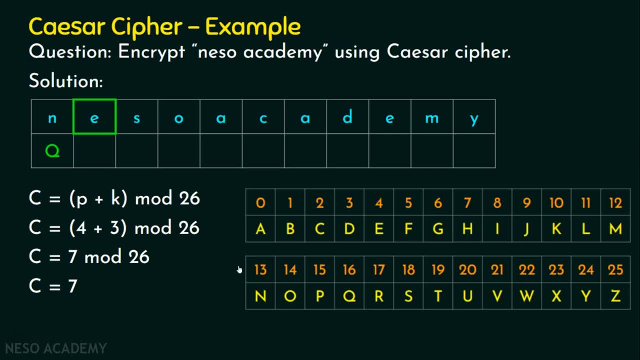 H. right, So E is encrypted as H. So the answer is H for this case. I'm going to place this H in the second place, which is this: Now let's encrypt the third one, which is S. 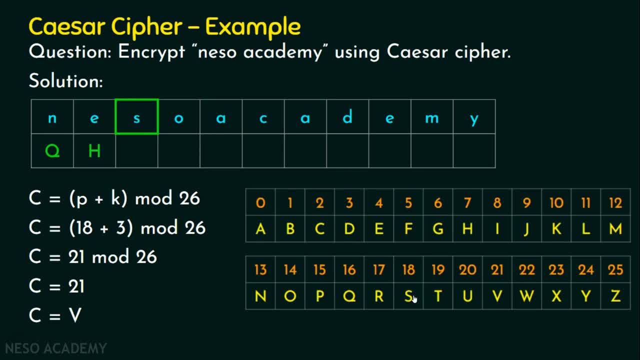 How can we do this? Very simple. What is the plaintext equivalent for S? It is 18, right, So 18 plus three mod 26,, which is 21 mod 26.. 21 mod 26 will give 21, and V is the equivalent. 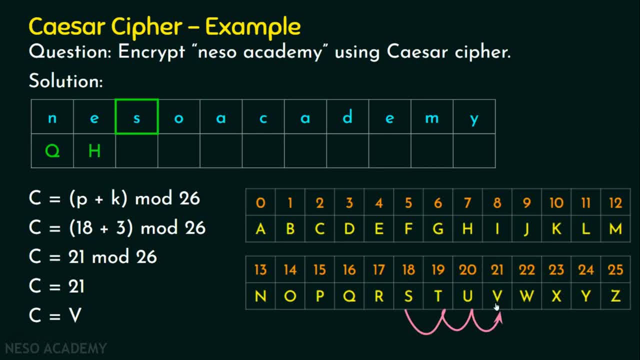 For 21,. what is the alphabet V? So V is the answer. We can also do this in simple terms. We know how many places we are going to shift. Three places right. So for S, the first place, the first shift, is T. 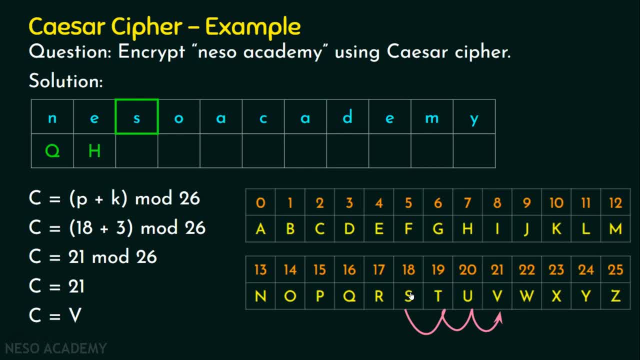 the second shift is U. the third shift is V. So S is encrypted as V. We need not go with this approach. If you are confident, you can use this direct approach. So S is encrypted as V. We can see: S is encrypted as V. 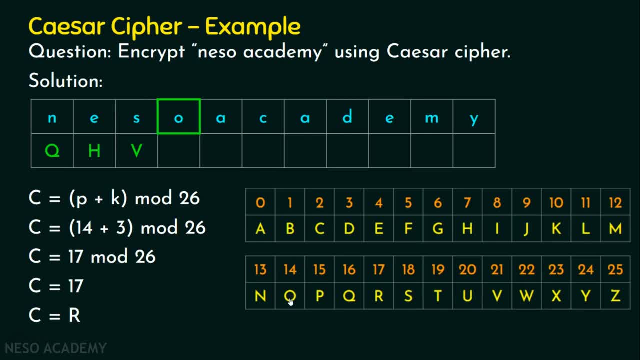 Let's take the next one, O. Let's see how O is encrypted, as This is the first shift, this is the second shift, this is the third shift, So O is encrypted as R, right, So you can take this approach also. 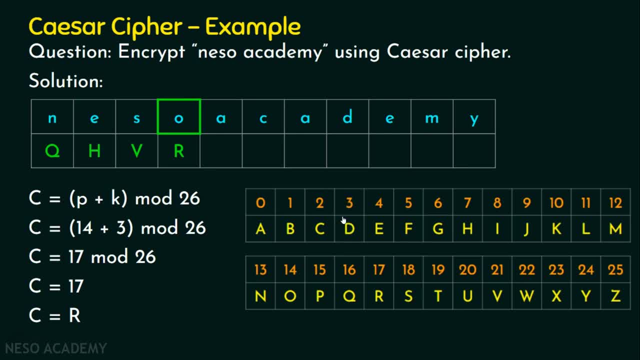 A is encrypted as one, two, three. So A is encrypted as D, C is encrypted as F. A is encrypted as D, C is encrypted as G. E is encrypted as H. M is encrypted as P And Y is encrypted as. let's solve this now. 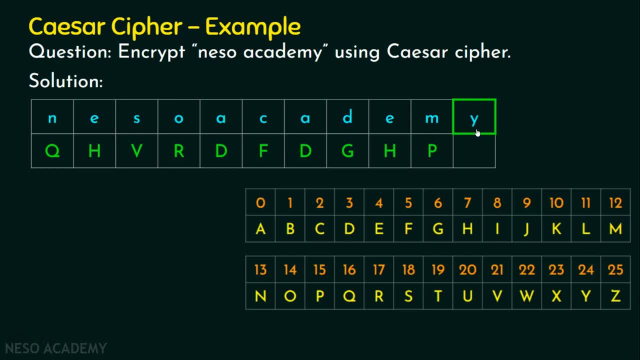 because we are going to see how mod is helping us to get the reminder. Say Y, how many shifts we are going to do Three shifts, right, This is the first shift, then wrap around, This is the second shift and this is the third shift. 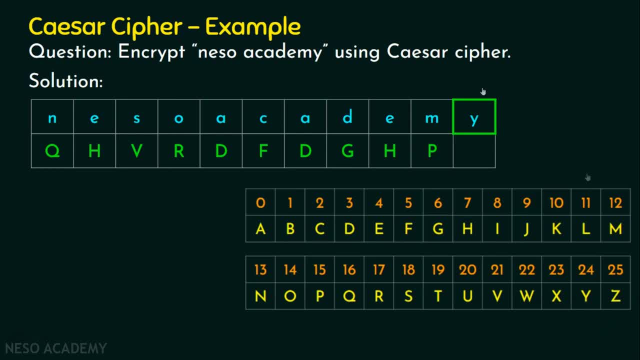 I repeat, for Y, this is the first shift, then this is the second shift and this is the third shift. So Y is replaced as B. Let's solve it using the equation approach. We know what is the letter for Y: it is 24.. 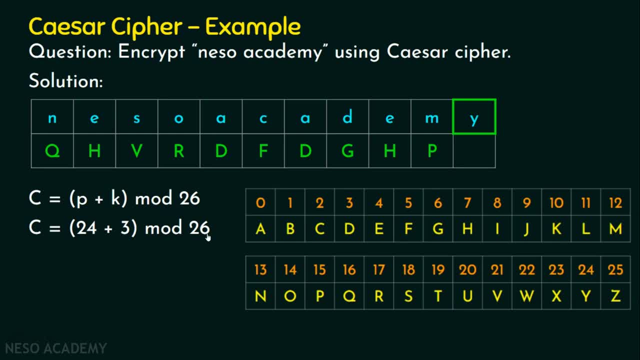 So 24 plus 3 mod 26.. 24 plus 3 mod 26 is equal to 27 mod 26.. We will divide it 27 when it is divided by 26.. 26, 1 times 26 and the remainder is 1.. 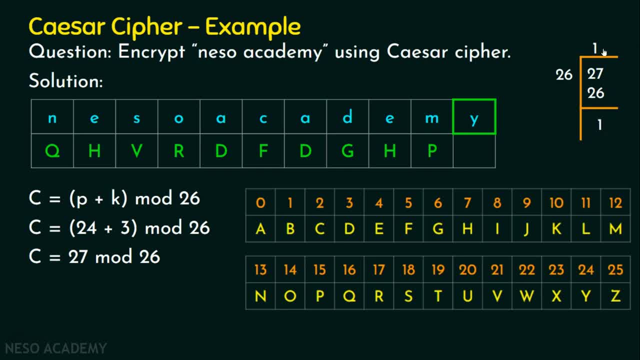 See, please note, we need to take this value only, not this value, Because in mod we should always take the remainder. What is the remainder for 27 mod 26?? It is 1.. What is the value present in 1 or alphabet present in 1?? 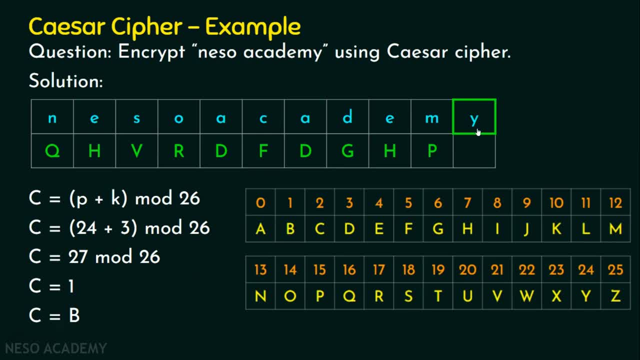 It is B, right, So the ciphertext for the plaintext letter Y is B. We can also do this simply: Y means the first shift Z, the second shift A and the third shift B. Since we are dealing with Caesar cipher, we need the key value as 3..